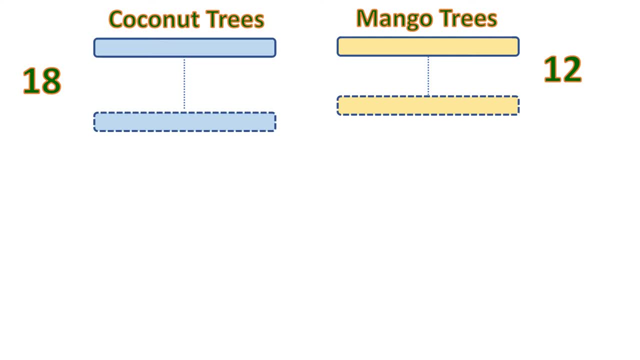 it is. it must be the same number of trees for each row and there are only 12 mango trees in all, so it must be lesser number of rows. and which one are we going to use? the least common multiple or the greatest common factor? so, based on the problem we are after of the biggest divisor that can divide both: 18. 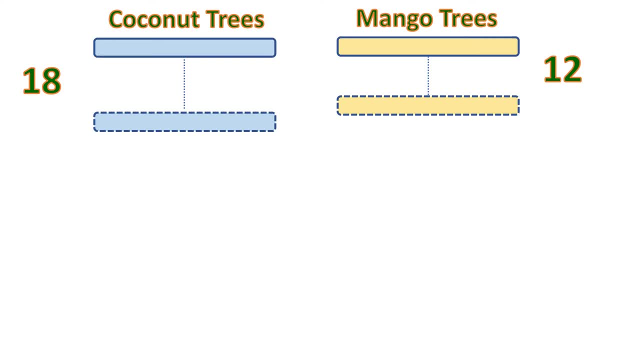 and 12, so that it will be the number, the same number of trees for both coconut trees and mango trees. and just inform, your greatest common factor is the same concept with the GCD, which is the greatest common divisor. so if you are looking for the greatest common 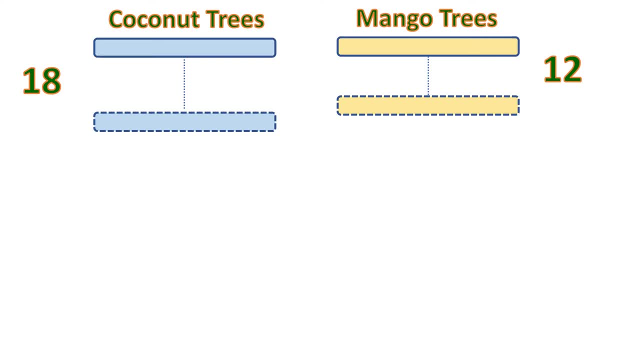 divisor, just like this, looking for a biggest divisor for both 18 and 12, that is. that means you need to use greatest common factor, or if you are unsure with the problem and if it involves asking for the greatest number, so probably it is asking you to do you find the greatest common. 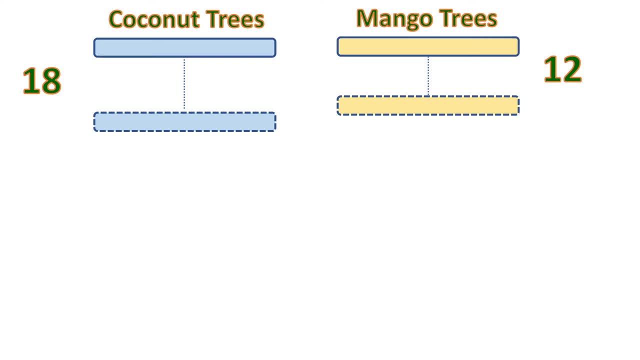 factor, but it is not always like that. so, but just in case you are not sure what to do, then just look at the problem it involves greatest, then probably it's greatest common factor. but still, the best way to do is to find, to understand the problem, so you will know what to use. so let's have, let's use the continuous. 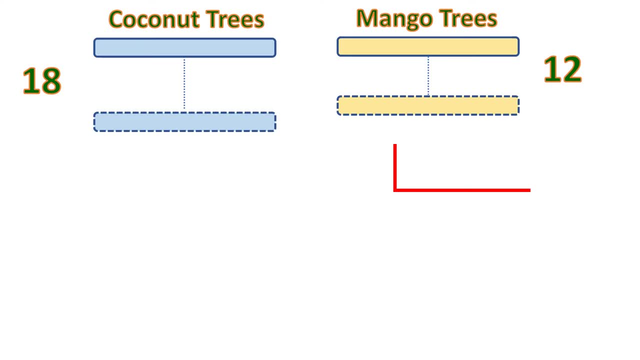 division to find the greatest common factor. so we have 18 and 12, and both are even numbers, so it can be divided by 2. so 18 divided by 2 is 9. 12 divided by 2 is 6. so let's continue to 9. and 6 are divisible by 3. so 9 divided by 3 is 3- 6. 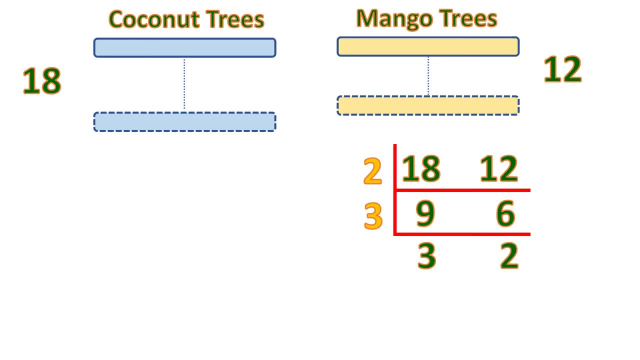 divided by 3 is 2, and so let's have now the greatest common factor. so I'm going to multiply those numbers the left. so 2 times 3, that will be 6, so there are 6 trees in each row. now let's have another problem. 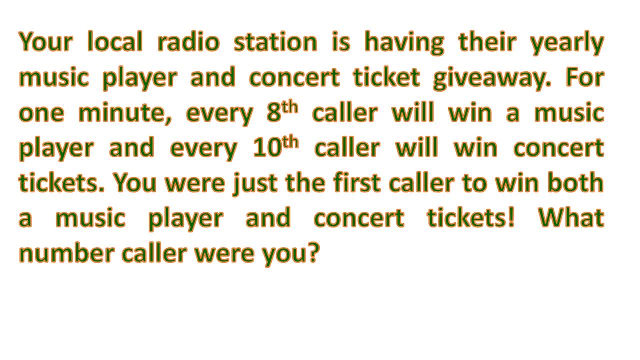 they have. your local radio station is having their yearly music player and concert ticket giveaway for one minute. every eight caller will win the music player and every tenth caller will win concert tickets. you were just the first caller to win both a music player and concert tickets. what number caller were? 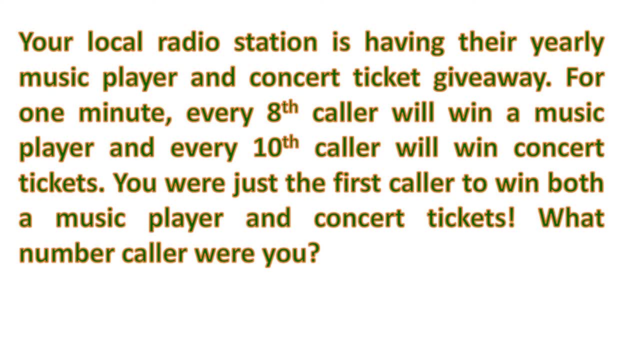 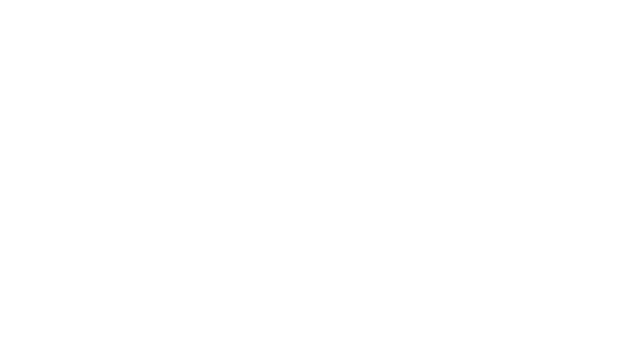 you. so let us try to understand the this problem and identify whether it is then falls greatest common factor or it involves least common multiple. so the problem is like this. so here's the for the music player and how you will win it. you will be the eighth color, next will. 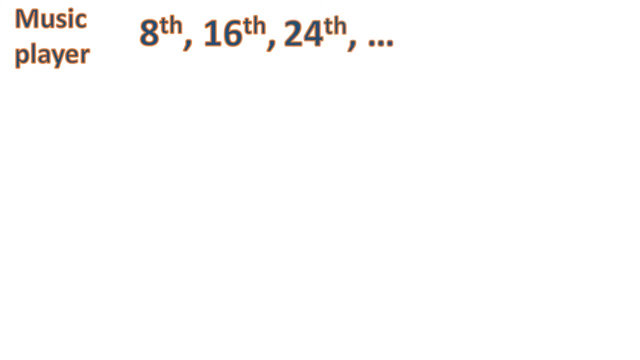 be 16th color, next will be 24th color, because it's gonna be every 8 and also for the concert ticket. so when you will win concert ticket, if you are the 10th color, and then after that if you are the 20th color and the 30th color now, since 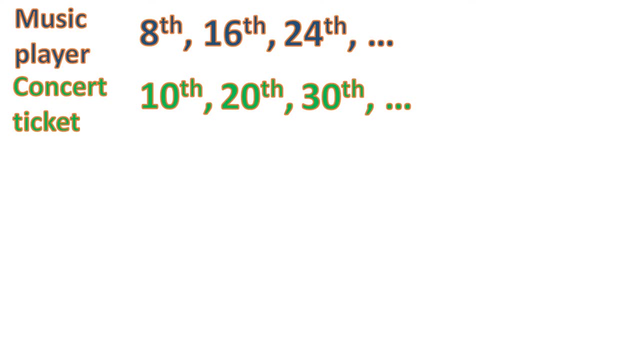 it's given that you have won both music player and the concert ticket. that means both it, but the the the time that you're called is, must be the same. it must be simultaneous for both music player and the concert ticket. now the question is: when did it happen? when did this meet the? the sequence for 8 and for the 10 and. 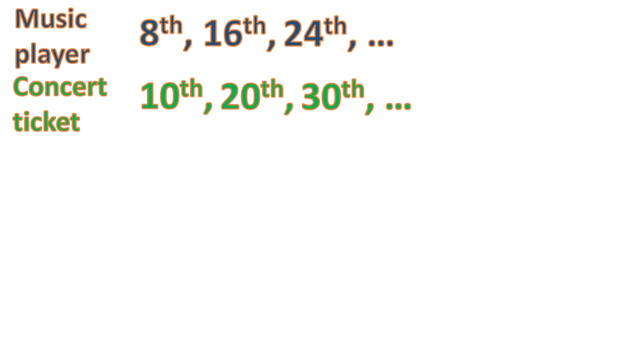 observing the see the problem. it is actually talking about multiple seconds of 8 and multiples of 10. so this involves least common multiple and so let's have, let's use the continuous division. so we have 8 and 10 and we're going to find the least common multiple of this problem. so 8 and 10 are. 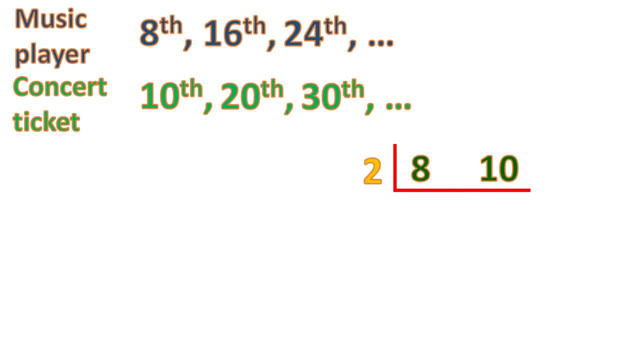 divisible by 2. so let's divide by 2. 8 divided by 2 is 4 and 10 divided by 2 is 5. now we have 4 and 5 and there's no common number to divide with 4 and 5. 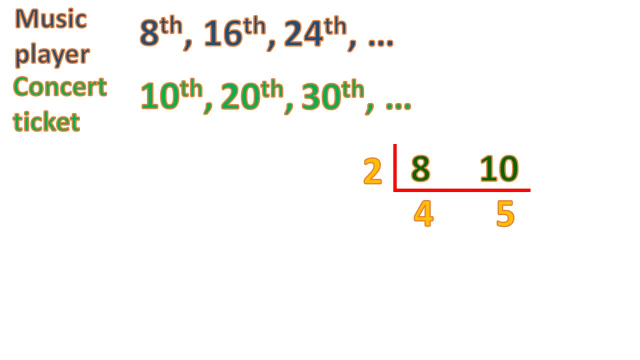 then we can have now the least common multiple or the LCM. so let's multiply. we have 2 times 4 times 5. so that's how you get the LCM. you by the left number and number at the bottom. so 2, 4 and 5, and product is 40. so 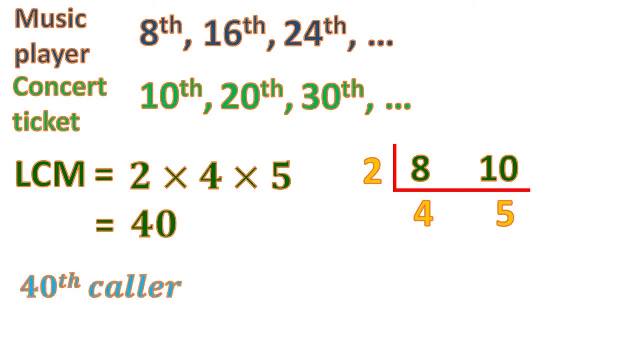 that means you are the 40th color. that's why you get both music player and the concert ticket. so the idea there is: you use LCM if it involves multiples, and if you are unsure which one to use, you will know if it's LCM if it involves multiples, and if you are unsure which one to use, you will know if it's. 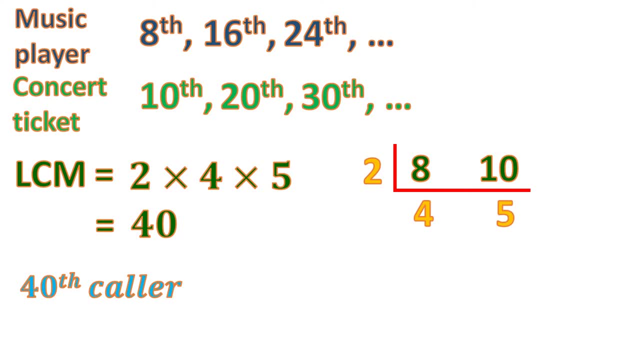 it involves LCM. if it's asking for something about the minimum number, for the least number or the smallest number, if it's a problem- it was like that- probably it's the LCM, although it's not always in that case, but most of the time. just in case you are unsure, but still, the best way to know which one to use is: 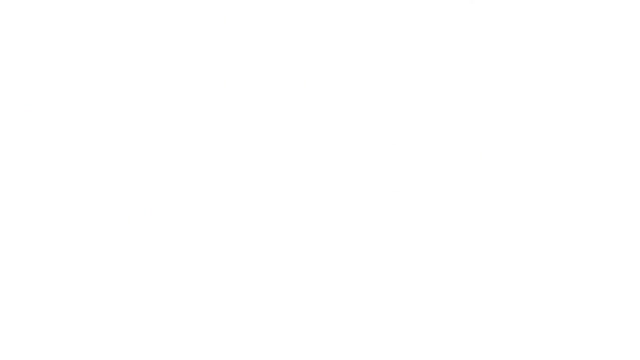 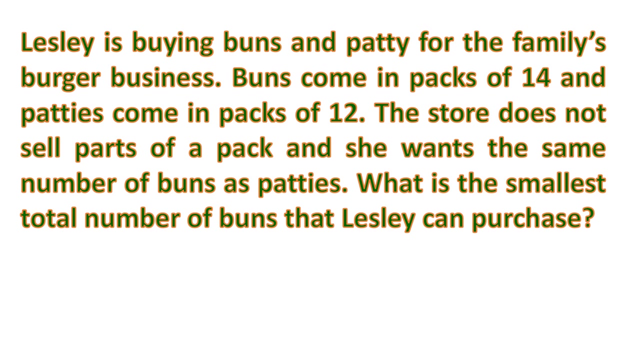 to understand the problem. now let's try to solve another problem problem we have. leslie is buying bonds on patty for the family's burger business. bonds come in packs of 14 and patties come in packs of 12.. the store does not sell parts of a. 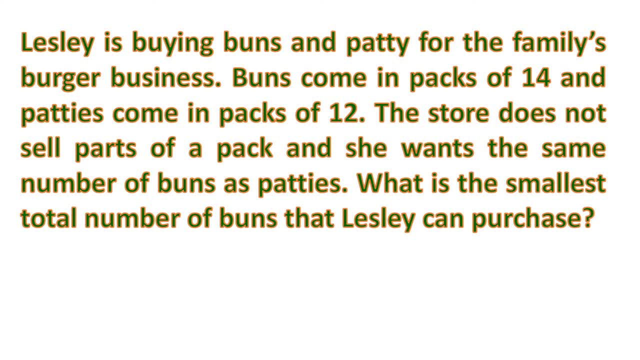 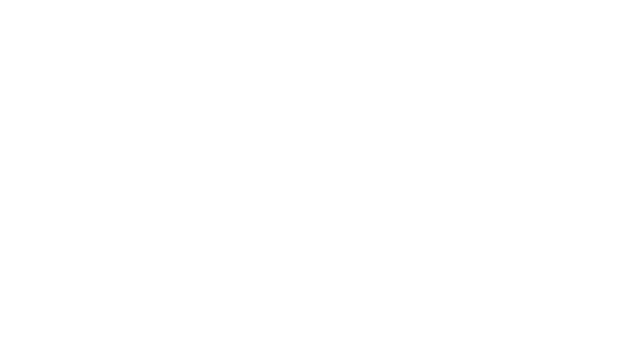 pack and she wants the same number of bonds as patties. what is the smallest total number of bonds that leslie can purchase? so let's analyze this problem. so let us look at how many bonds for each pack and how many patties for each pack. so for one, one pack will be 14. if there will be two. 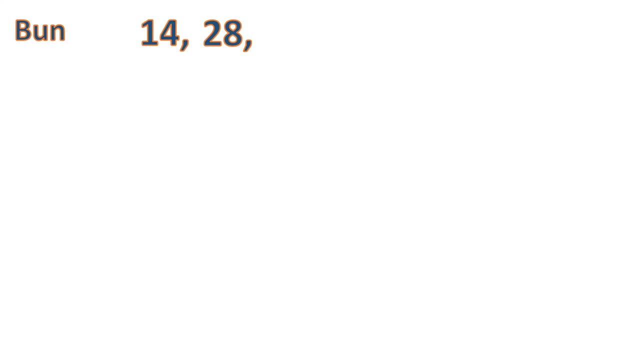 packs, then it's gonna be 28. if there are three packs to buy, then that's gonna be plus 14, which will be 42, and so on. for the patties, there are 12 patties for each pack. if we're gonna buy two, then they're gonna be 12 plus 12 is 24.. 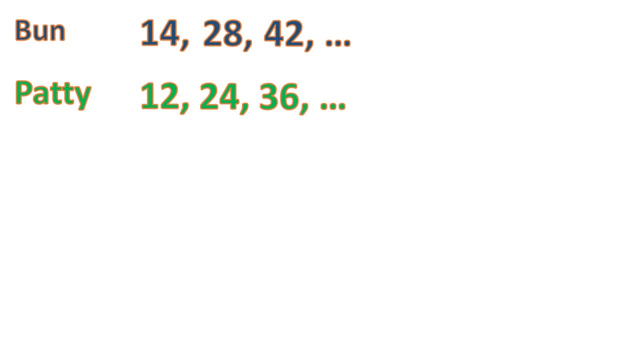 if i buy three packs, then it's gonna be 36 packs, and so on, and leslie wants to buy, such that the number of bonds and number of patties must be the same, and that's what we are looking for. when will this be? the sequence, the same? so observe that it is. 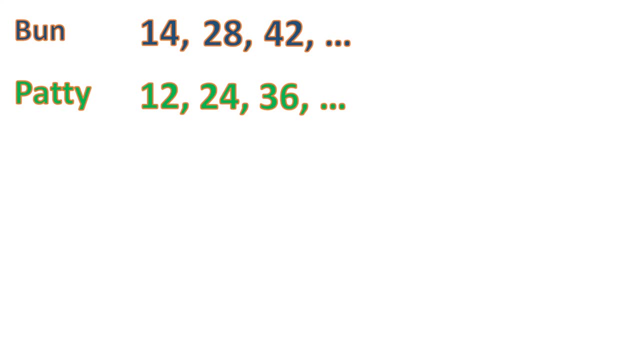 uh, involving multiples of 14 and 12.. so that means it's looking for the least common multiple, and so let's use continuous division, or you may use actually listing or prime factorization, so it will be up to you, but for me i i see it like the continuous division is the easiest way to do. 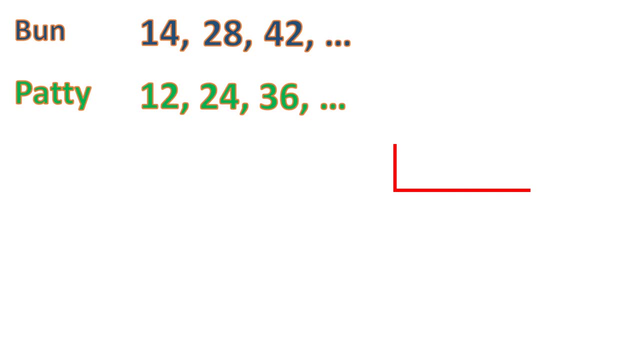 lcm and or gcf. so let's put 14 and 12 and divide. these are numbers. so let's divide by 2. 14 divided by 2 is 7. 12 divided by 2 is 6. then let's find the LCM. so let's multiply all three numbers we have 2 times 7 times 6 it. 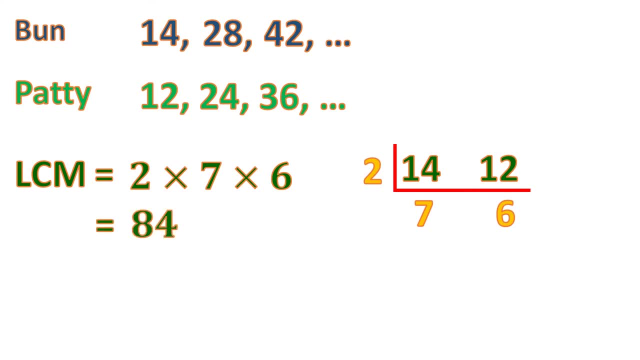 will be 84. so if we keep on adding packs of bonds then it's gonna reach 84, as well as the patties. so we are not sure how many packs are there for bun and patty, but we are sure that at some point it will be the same number of buns and 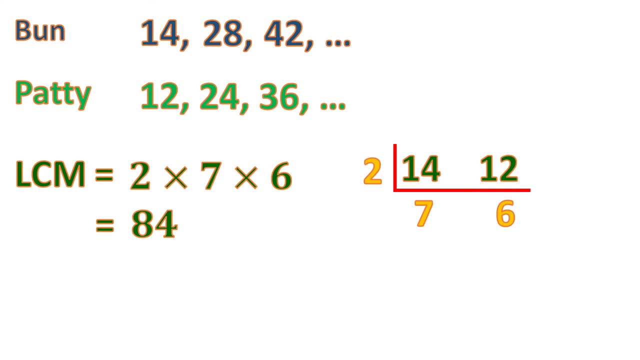 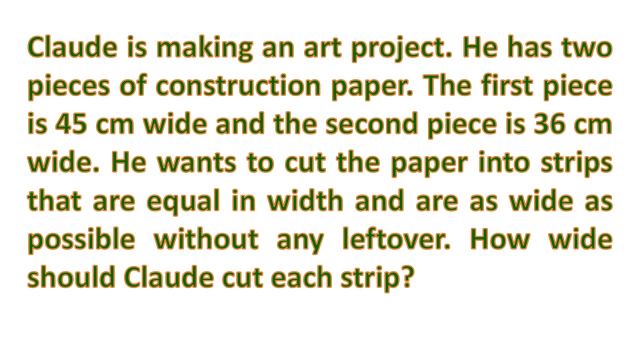 patties. so there's gonna be 84 by bonds and patties. but the problem is asking for the bonds, so there will be 84 bonds. so let's take another problem. Claude is making an art project. he has two pieces of construction paper. the first piece is 45 centimeters wide. 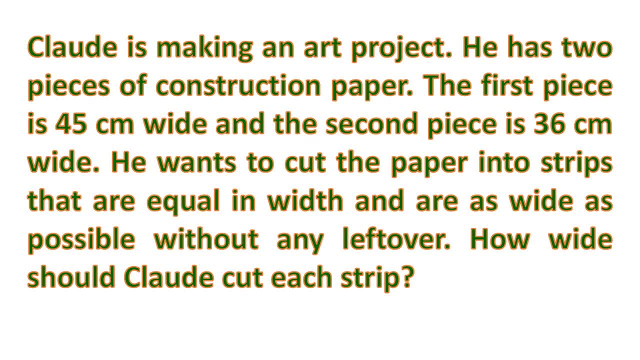 and the second piece is 36 centimeters wide. he wants to cut the paper into strips that are equal in width and are as wide as possible without any left over. how wide should Claude cut each strip? so let us try to solve this. so let's illustrate the problem. 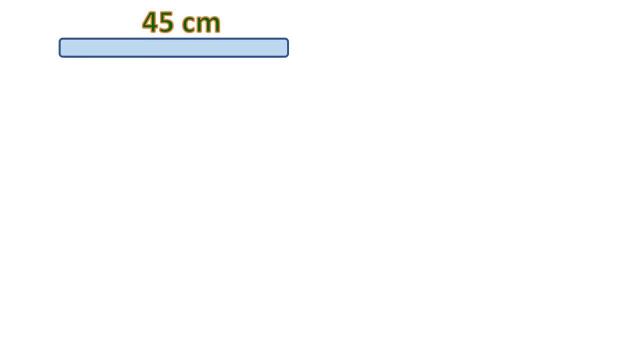 so we have this for 45 centimeters and 36 for 36 centimeters. of course it must be shorter, but of course this is not drawn to scale. so our problem is to look for to divide this into strips where it will be the longest, but it must be. 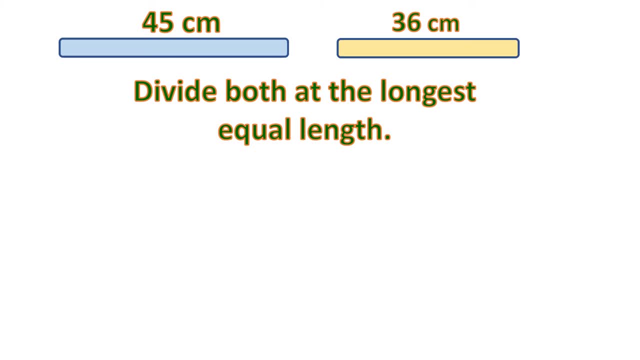 at equal length. so of course this involves dividing and it involves the greatest, and because from the word longest it can be the greatest, and from the word equal it's mean, it means common. so you're looking for the greatest common divisor, so it's looking for the greatest or the biggest number that can divide both 45 and 36. so it involves gcf or greatest common factor. so let's solve this. we have 45 and 36 and we're going to divide it, so both are divisible by 3.. so 45 divided by 3 is 15.. 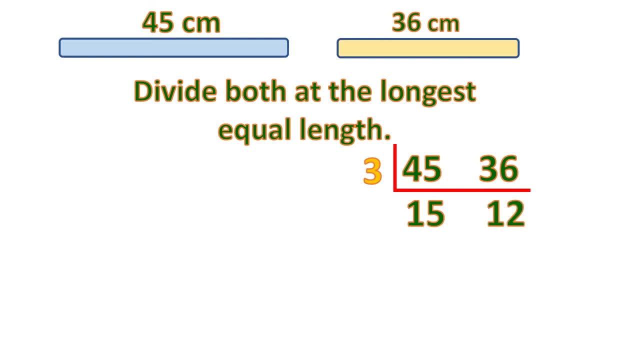 36 divided by 3 is 12.. then let's continue dividing. 15 and 12 are both divisible by 3. again, 15 divided by 3 is 5. 12 divided by 3 is 4.. you're solving for gcf. you just multiply the numbers at the left. 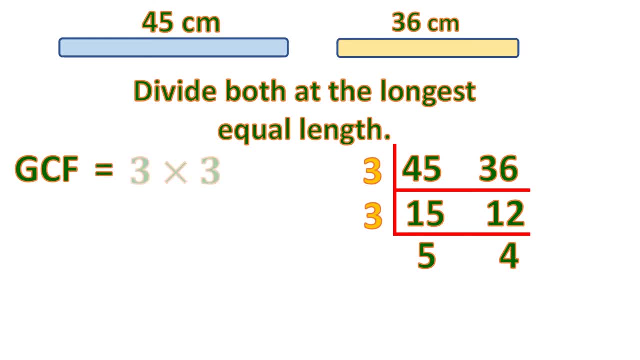 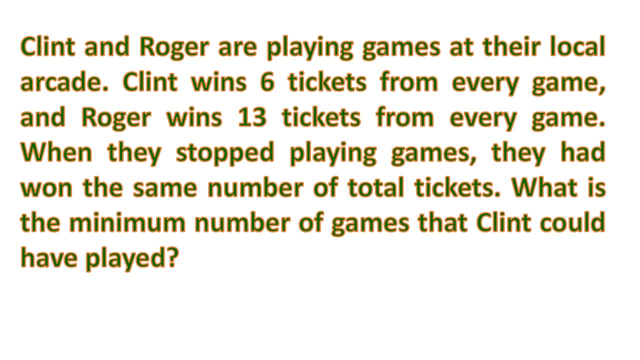 so let's get the gcf, which is equal to 3 times 3, that is 9.. so the answer is 9 centimeters wide. so let's take another problem we have. Clint and Roger are playing games at their local arcade. Clint won wins six tickets for. 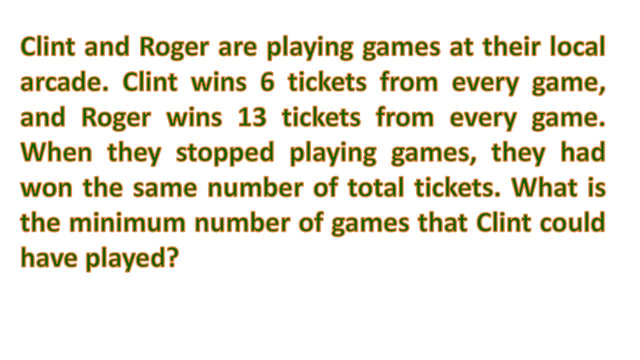 from every game and Roger wins 13 tickets from every game. when they stopped playing games, they had won the same number of total tickets. what is the minimum number of games that Clint could have played? so we actually don't know. so the given is they're both playing game. we don't know what game it is, but you. 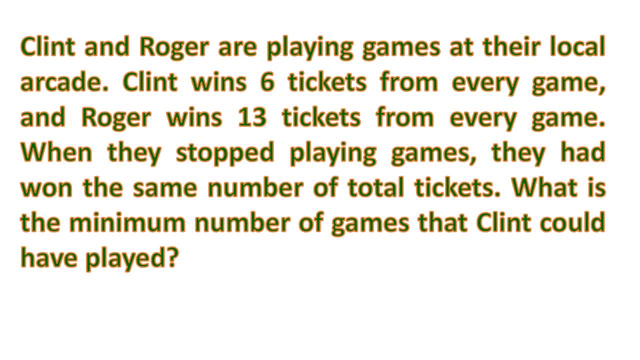 are sure that for every game Clint wins it's going to be six tickets, and Roger for every win in in his game it can be 13 tickets. but after playing the game we don't know how many games they have played, but at the end of their their game they have the same number of tickets. 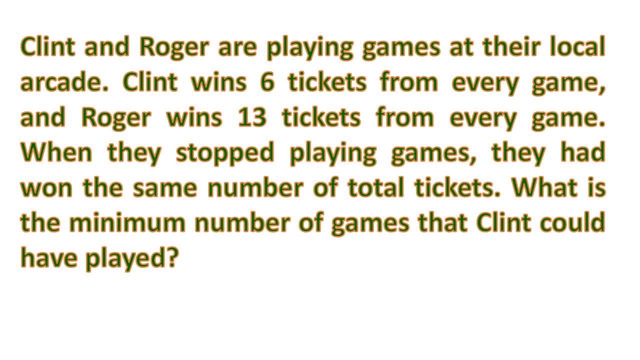 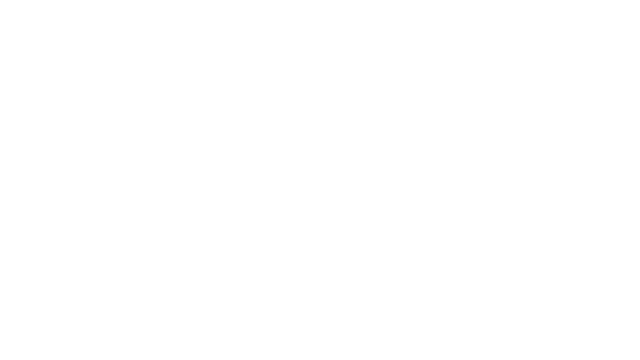 so there are many possible ways to have number of the same number of tickets, but it is looking for the minimum number of games because there are so many possible number of games, so it's only it's asking for the minimum number of games that Clint could have played. so let us solve this. 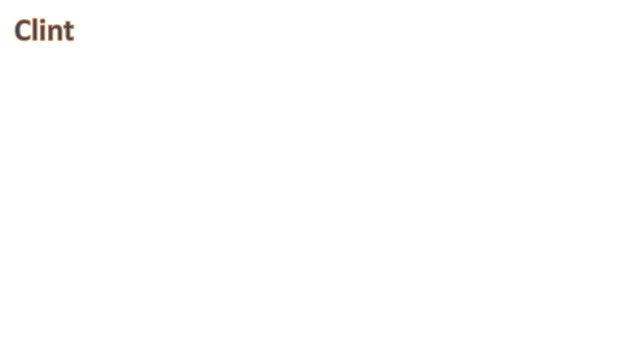 so to let us illustrate the problem. so Clint will win for every game with six tickets, and if you will play another game plus six is 12 tickets and another game plus six, it will be 18 tickets. for Roger. for the first game, he will get 13. 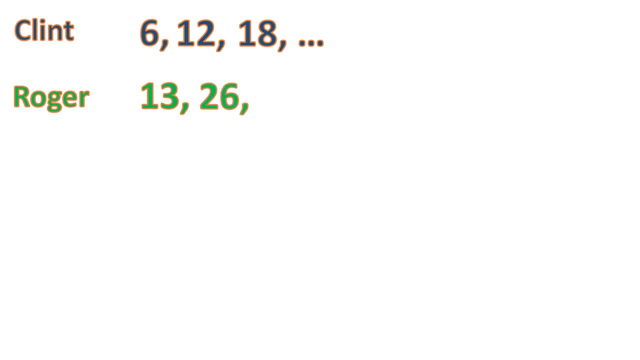 tickets. another game plus 13 is 26. another game is 39 tickets. so the problem is asking for the number of games played by Clint. but before you can solve that you need to know how many tickets are there in where they have the same number of tickets. 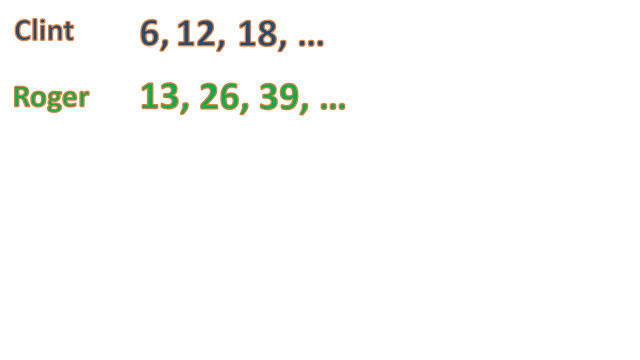 so problem is asking when this six becomes the same as number of multiples of 13.. so it involves a multiples of 6 and 13 and we're going to look for the smallest number where they have the same multiple. so, in short, it's asking for the least. 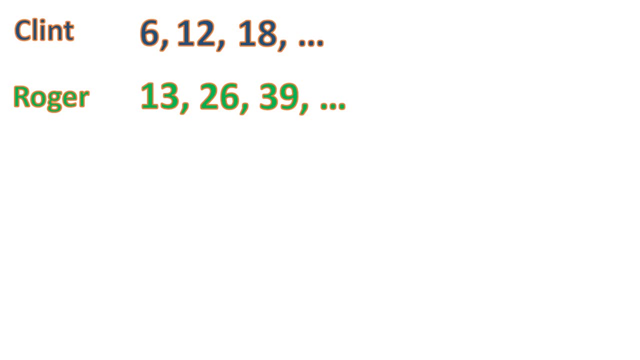 common multiple, so let's use continuous division for this. we have 6 and 13.. now 6 and 13 are the same, and 13 doesn't have the same and doesn't have a common divisor, so what you will do is just multiply them directly. 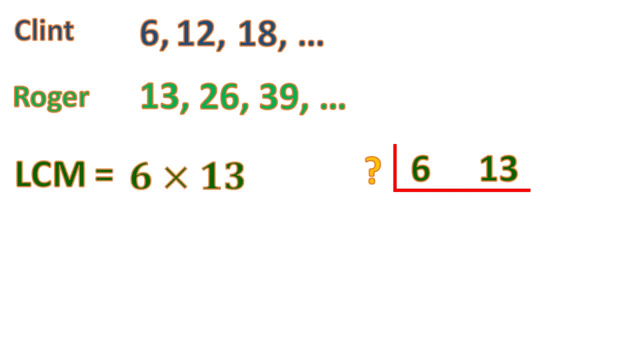 so the LCM is equal to 6 times 13, which is equal to 78 tickets. this means they could have 78 tickets. of course, there are other possible number of tickets where they will have the same, but we are looking for the smallest possible and so let's continue solving, because it's asking. 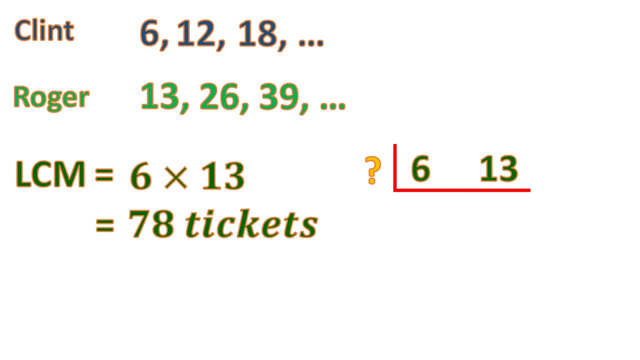 for the number of games played by Clint. it's not asking for the number of tickets, so let's only solve for 10. so 78 divided by 6, because it's 6 tickets for every games played. so 78 divided by 6 is 13.. so this means: 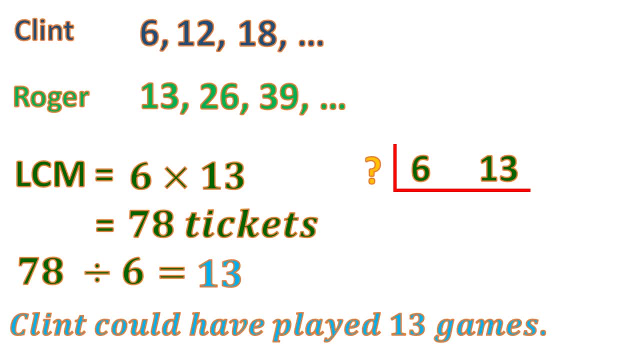 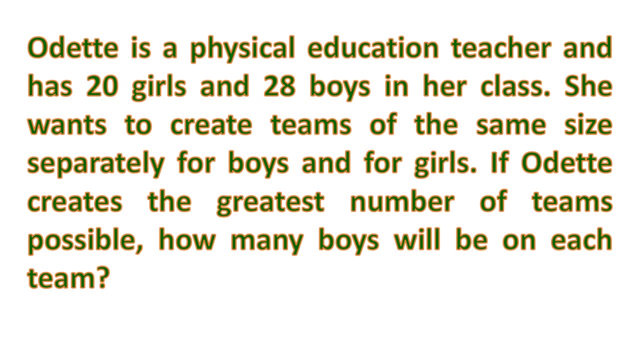 Clint could have played 13 games. so another problem. Odette is a physical education teacher and has 20 girls and 28 boys in her class. she wants to create teams of the same size separately for boys and for girls. if Odette creates the greatest number of teams possible. 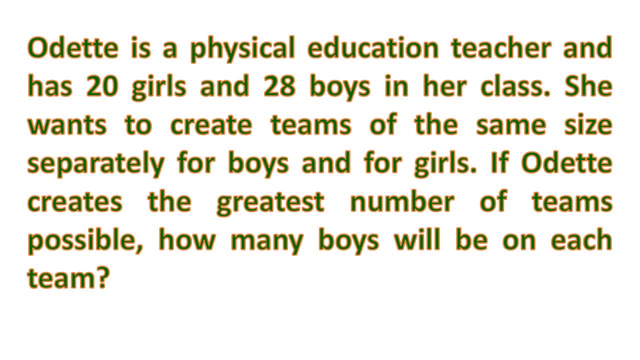 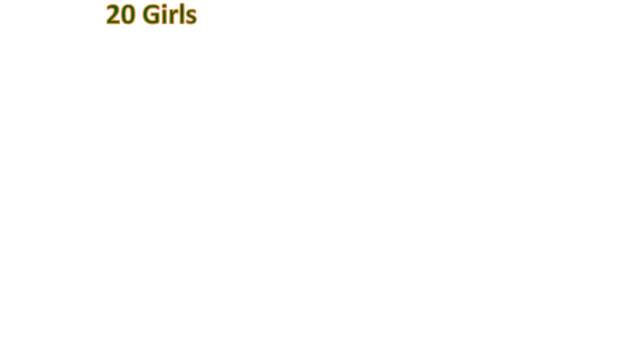 how many boys will be on each team. so let's analyze and solve this problem. so this is for the 20 girls, and we have this. I represent every girl with a with a pink box, and for 28 boys, I represent every boy with blue box, and the problem is asking for. it involves 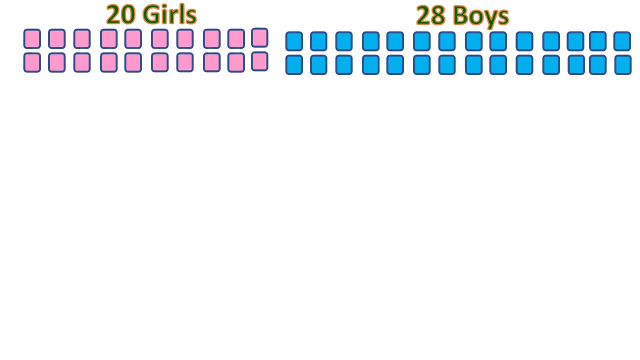 division of this number of girls and number of boys, where Odette wants to maximize the number of members for every group and it not. it is not necessarily the same number of girls and number of boys for every group, as long as it is the same within the group of girls and it's the same. 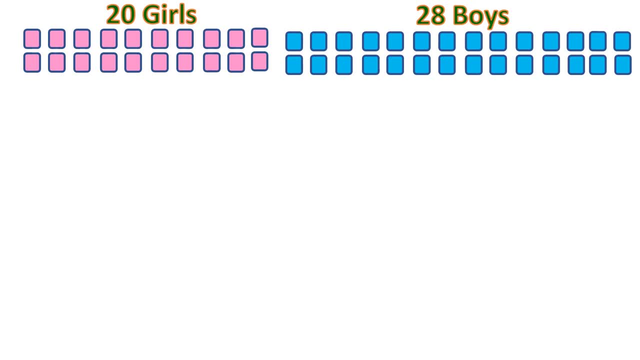 within the group of boys. okay, so, as you observe, as you analyze the problems, it is something involving the divisor, the biggest divisor for both boys and girls. so it must be involving the divisor, the biggest common factor. so let's use continuous division. we have 20 and 28, so let's divide. and these are even numbers, so let's. 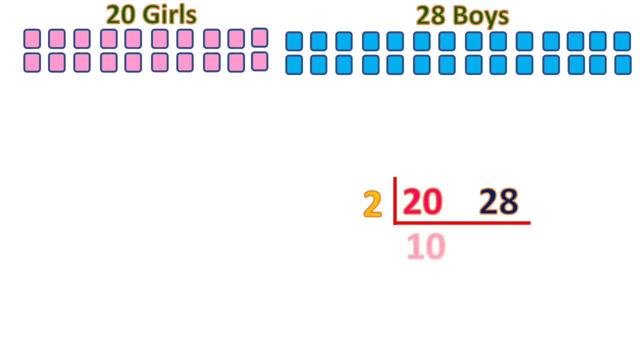 divide by 2.. so 20 divided by 2 is 10, 28 divided by 2 is 14, and these are even numbers. so let's divide this by 2. 10 divided by 2 is 5, 14 divided by 2 is 7.